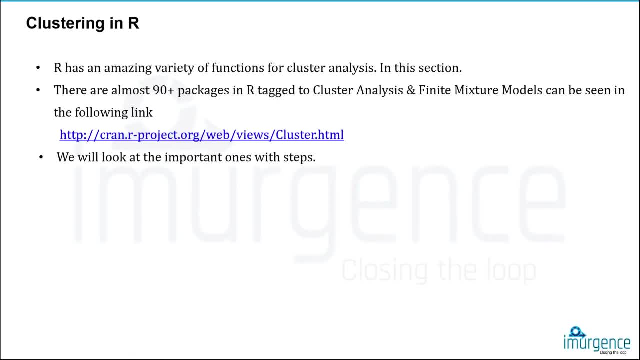 So clustering in R, so you have different algorithms, and in R to do anything, you have more than 20 package basically. So there are almost 90 plus packages in R for cluster analysis and finite mixture models. So obviously you can understand that there are so many and we'll be using one of. 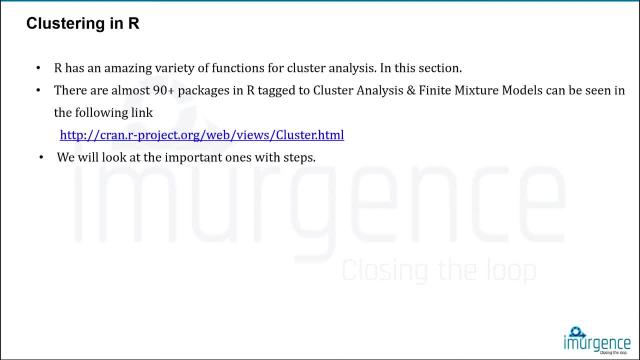 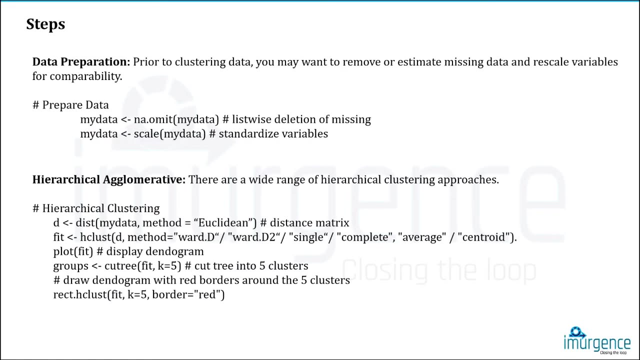 the very basic which comes with base R, which is k means k with a small k, and there is obviously a k with a capital K also, which is present in the AMAP package. We won't be using that. we'll be using the small k means package. So let's look at the important steps. So now, first of all, you have 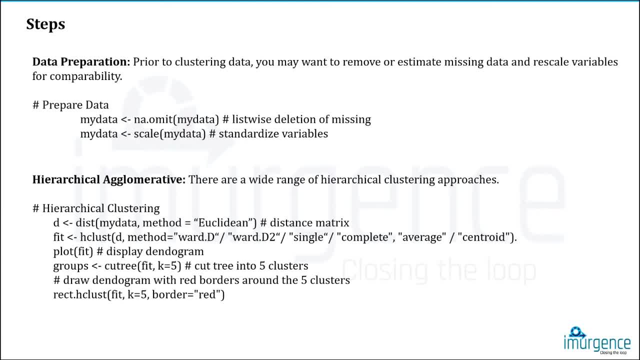 to prepare your data. So you will be removing empty values, that is, any values- from your data, right? So what you are seeing on the screen is just an empty shell structure. Later on, we'll be doing that with the hands-on also, right? So you will extract the data. you will save it somewhere. 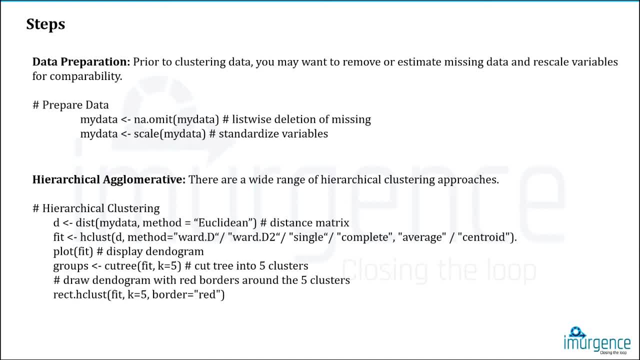 and you will be able to do that. So you will be able to do that with the hands-on also, right? So then you will remove the any values from that, you will standardize the data by means of scaling so that all the dimensions are given equal importance, and then we'll step into hierarchical. 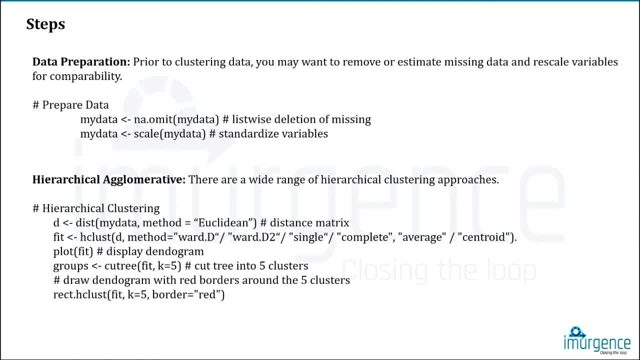 agglomerative clustering. So it goes by: you'll select an object name, allocate first. create the distance metric by using the Euclidean method. use the hcluster package to actually create the clustering model, save it with some name and then you can use the. 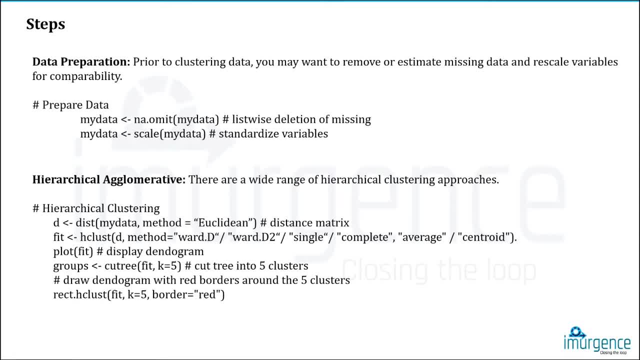 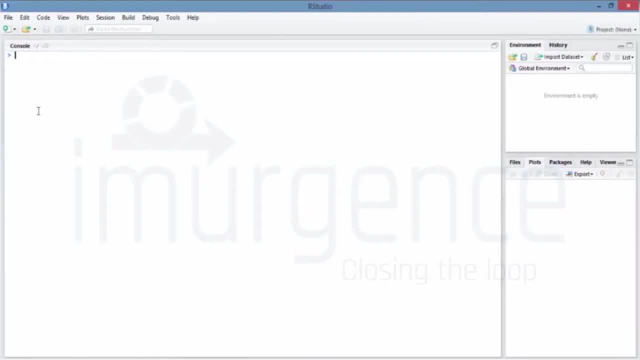 for a plot, so you can plot this model right and then you can use this to cut your data into five different clusters. we'll be just using some existing data, so let's say the slide previous to this. okay, so I'm saying: require data sets. I'm just loading this: data sets right and 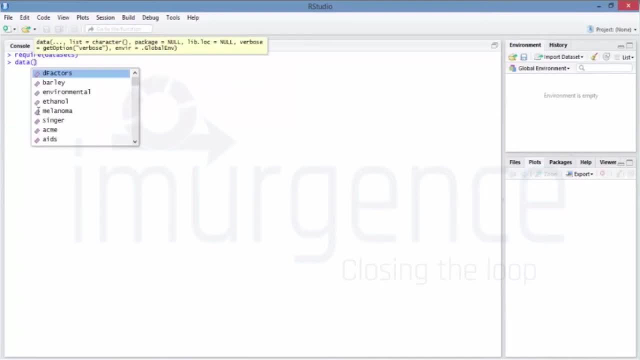 I'm saying data, so you have the USA RS data. okay, fine, and I'm using a variable name called as USA, in which I'm using the US data, and I'm using a variable name called as USA, in which I'm using the US data and I'm using a variable name. 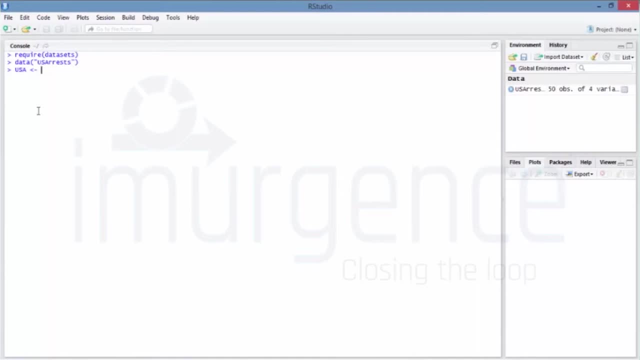 which I'm saving this data again. but I'm doing something like an any dot omit, which I'm saving this data again. but I'm doing something like an any dot omit because we know that if you use an any dot omit, it will isolate the n is and 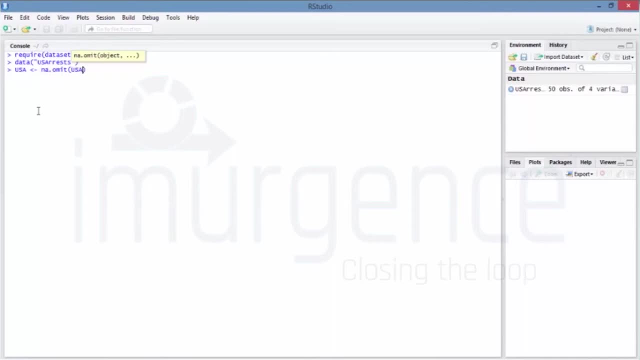 because we know that if you use an any dot omit, it will isolate the n is and delete the whole rows. where in any data is present right, so it will remove the. delete the whole rows where in any data is present right, so it will remove the data where, if you have an any, it will isolate that and remove it. now you can. 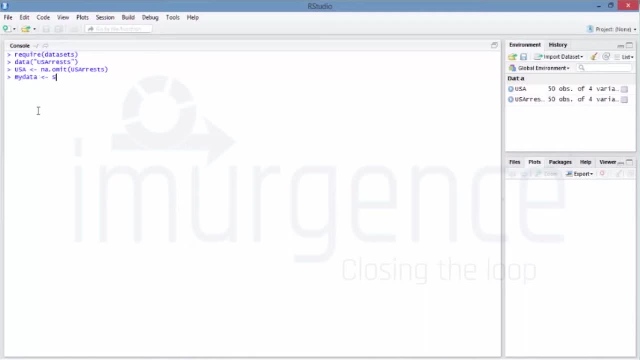 data where, if you have an any, it will isolate that and remove it. now you can save this as my data and just do some transformation. so we are going to scale, save this as my data and just do some transformation. so we are going to scale the data. 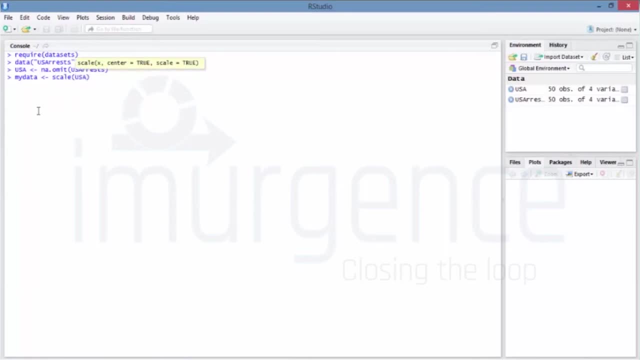 the data. so I'm going to scale it using the scale functionality. wait so you have. so I'm going to scale it using the scale functionality. wait, so you have done the scaling part. now you will be using the hierarchical clustering. so I'm done the scaling part. now you will be using the hierarchical clustering, so I'm 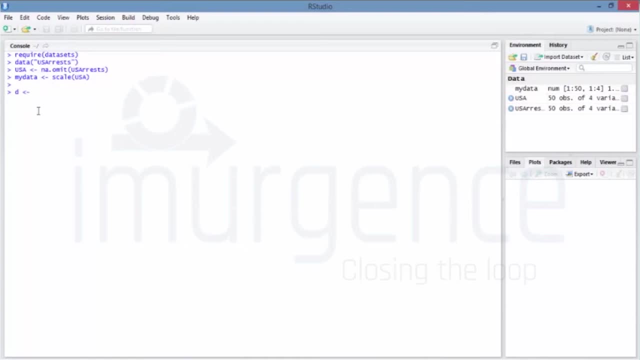 going to create a variable called say. going to create a variable called say. going to create a variable called say, supposedly D, in which I'm saying supposedly D, in which I'm saying supposedly D, in which I'm saying allocation distance. so I'm computing the allocation distance, so I'm computing the. 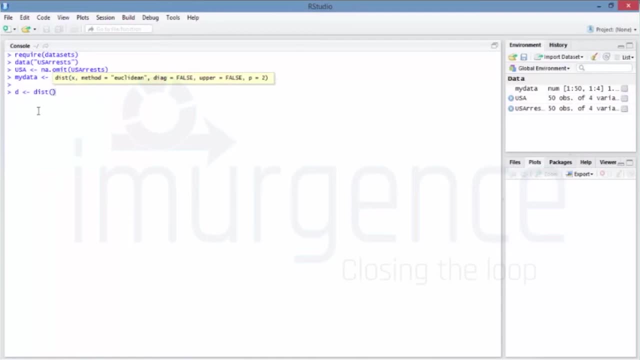 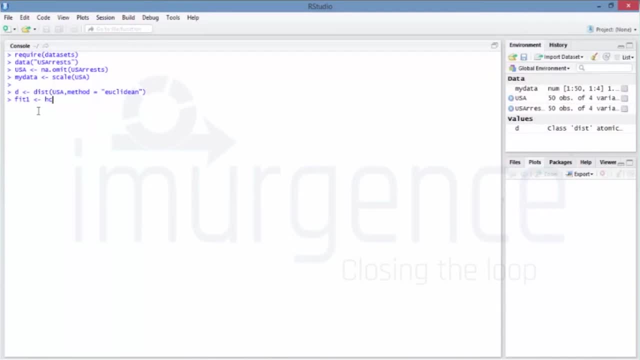 you Lydian right, so you fit one allocation sign H class. so I'm running different sign H class. so I'm running different sign H class, so I'm running different iterations and that I'm passing the iterations and that I'm passing the iterations and that I'm passing the distance. matrix method is equal to board. 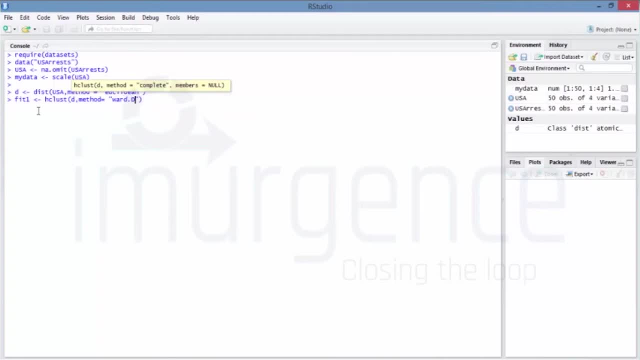 distance matrix method is equal to board. distance matrix method is equal to board. dot these. we have different methods dot these. we have different methods dot these. we have different methods which are already available. if you saw which are already available. if you saw which are already available. if you saw the linkage function, we had seen the 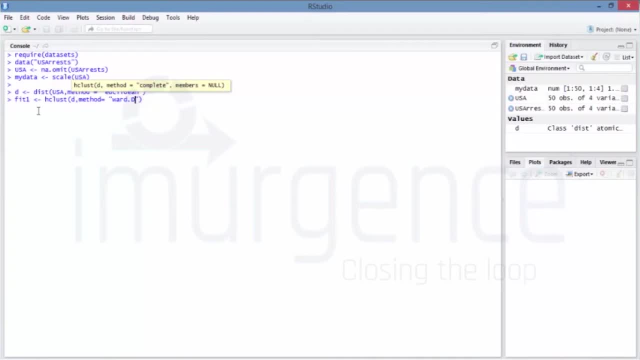 the linkage function. we had seen the, the linkage function. we had seen the single complete average centroid approach, single complete average centroid approach. single complete average centroid approach and all those things. so these are the and all those things. so these are the and all those things. so these are the various approaches which are present. so various approaches which are present. so, various approaches which are present, so you can refer to the head file, where you can refer to the head file, where you can refer to the head file, where you'll be getting the list of the same, you'll be getting the list of the same. 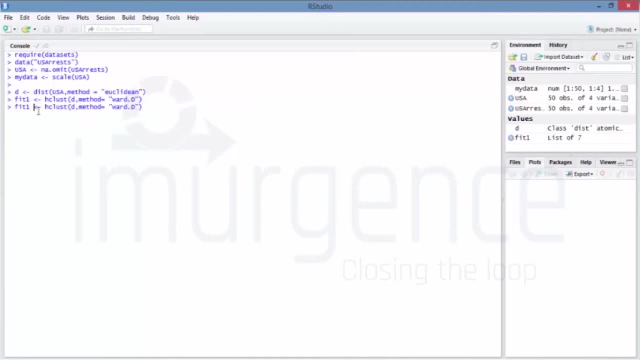 you'll be getting the list of the same. so I'm just going to run this quickly. so I'm just going to run this quickly. so I'm just going to run this quickly with the fit one to fit six, so that I'm with the fit one to fit six, so that I'm 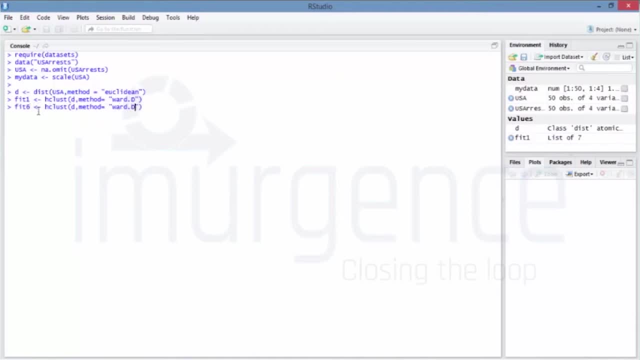 with the fit one to fit six, so that I'm just going to change these options and just going to change these options, and just going to change these options, and the rest of the things remain the same. the rest of the things remain the same. the rest of the things remain the same. so, from what be, I'm going to d2, then I'm 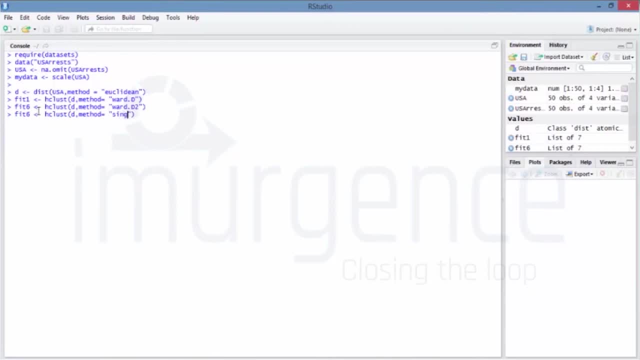 so from what be? I'm going to d2, then I'm. so, from what be I'm going to d2, then I'm saying single. I'm going to save it in saying single. I'm going to save it in saying single. I'm going to save it in fit, okay, I'm just. I have just renamed. 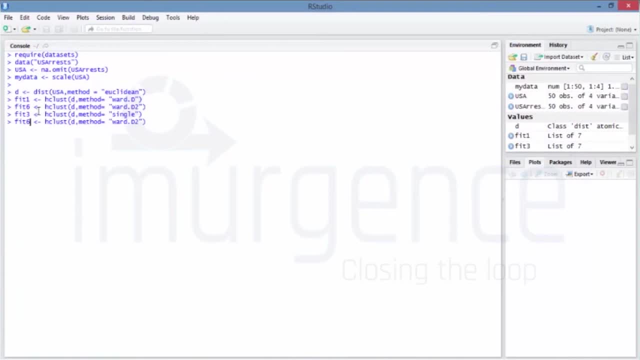 fit. okay, I'm just, I have just renamed fit. okay, I'm just, I have just renamed the previous one with the d2 on fit six, the previous one with the d2 on fit six, the previous one with the d2 on fit six and this renaming that to two. okay, so, 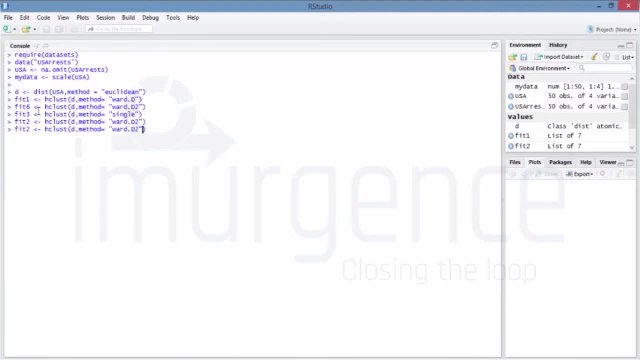 and this: renaming that to two: okay so, and this: renaming that to two: okay so. fit one. fit two. three is done now. we'll fit one. fit two. three is done now. we'll fit one. fit two. three is done now. we'll be doing it for fit four, and in this: 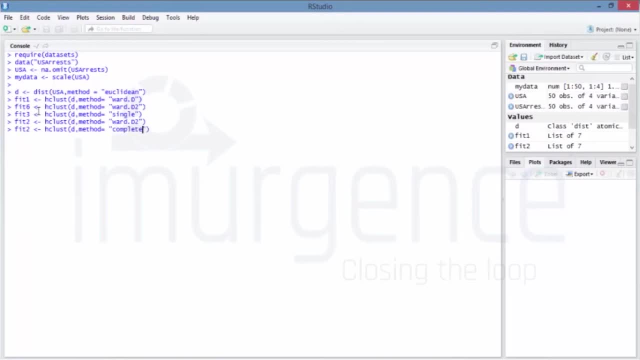 be doing it for fit four and in this be doing it for fit four. and in this case we are saying the complete linkage case. we are saying the complete linkage case, we are saying the complete linkage function and rename the object as fit function and rename the object as fit. 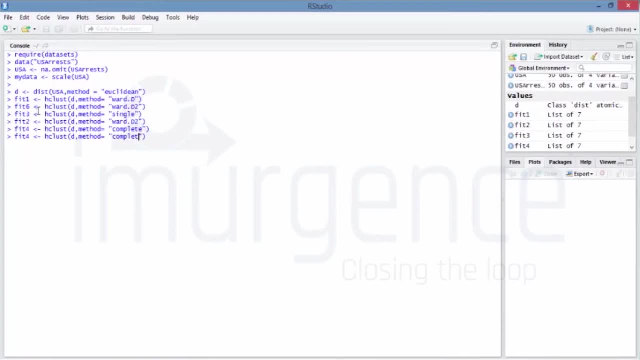 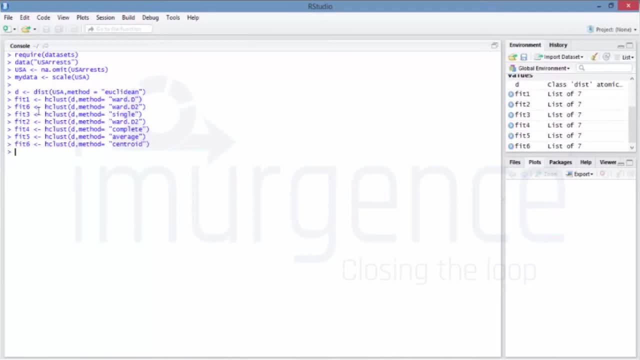 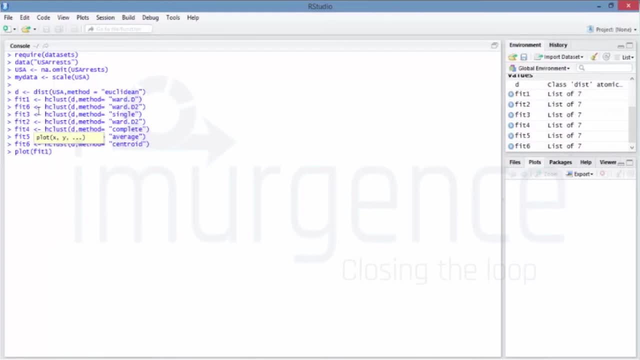 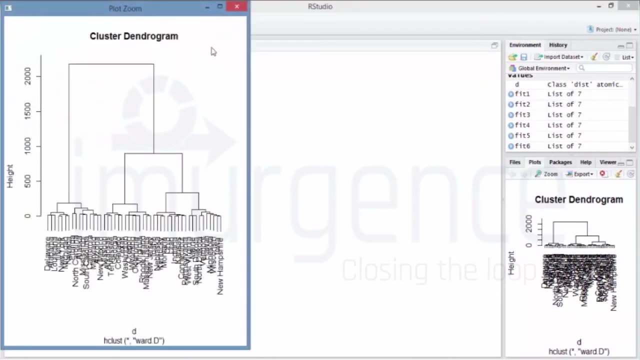 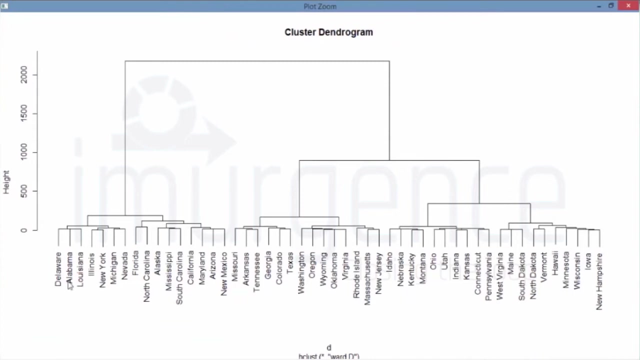 the six. so now let's plot these to have a look over here. so plot fit one. you have a look over here, so plot fit one. you have a look over here, so plot fit one. you can see the dendrogram over here. can see the dendrogram over here. 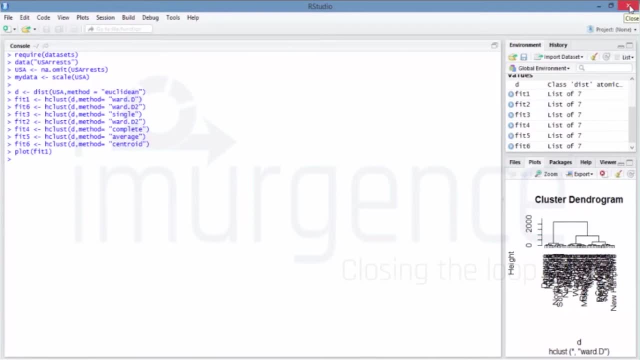 can see the dendrogram over here. so obviously you are not aware of the data, so obviously you are not aware of the data. so obviously you are not aware of the data. so you won't really directly, so you won't really directly, so you won't really directly understand this. but this makes sense if 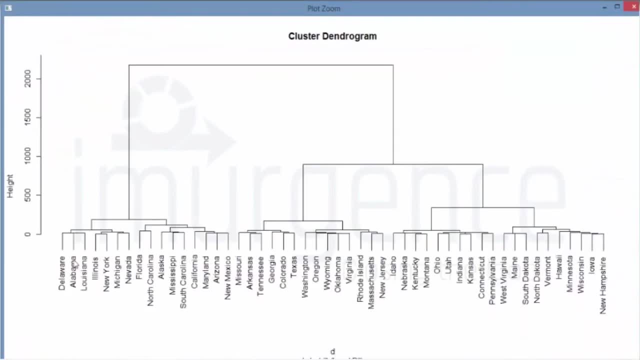 understand this, but this makes sense. if understand this, but this makes sense. if the data is small, if it is very huge, the data is small. if it is very huge, the data is small. if it is very huge, then it doesn't make sense, so these are. then it doesn't make sense, so these are. 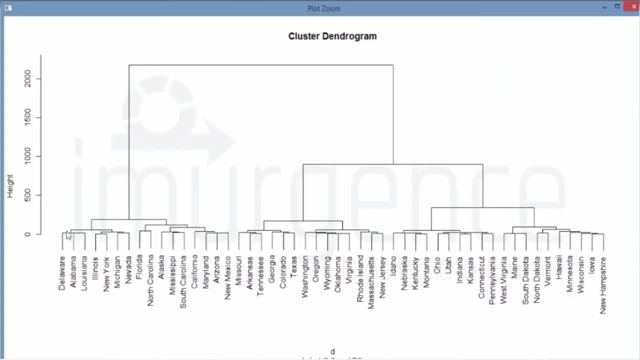 then it doesn't make sense. so these are the outcomes that the state have been, the outcomes that the state have been, the outcomes that the state have been. all these things given at different, all these things given at different, all these things given at different levels of height. so say, at this specific 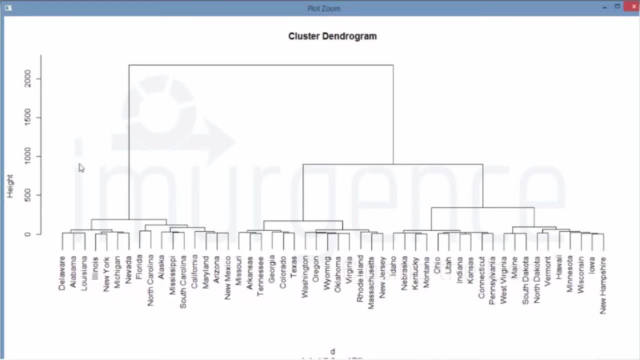 levels of height. so say at this specific levels of height. so say at this specific level. you can see that if people who are level, you can see that if people who are level, you can see that if people who are from this height, then there is a rule. 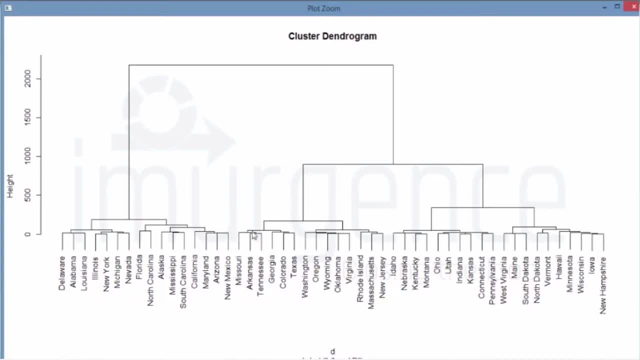 from this height, then there is a rule from this height, then there is a rule: again and then again. if the height is again, and then again. if the height is again, and then again. if the height is this much, if the height is this much, then this much. if the height is this much, then 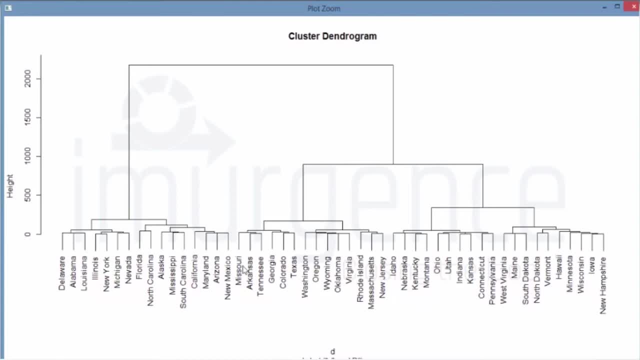 this much. if the height is this much, then, specifically, a person is from Missouri. specifically a person is from Missouri. specifically, a person is from Missouri. that's what you can draw as a conclusion. that's what you can draw as a conclusion. that's what you can draw as a conclusion. so I'm just going to close this and so I'm just going to close this, and so I'm just going to close this and further process this. so what you're further process this, so what you're further process this, so what you're going to do now is you're just saying. going to do now is you're just saying: 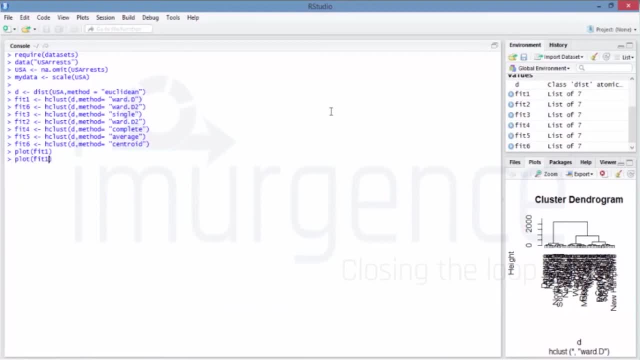 going to do now is you're just saying groups, or you can keep on doing the lots groups, or you can keep on doing the lots groups or you can keep on doing the lots will be a little bit of difference in will be a little bit of difference in. 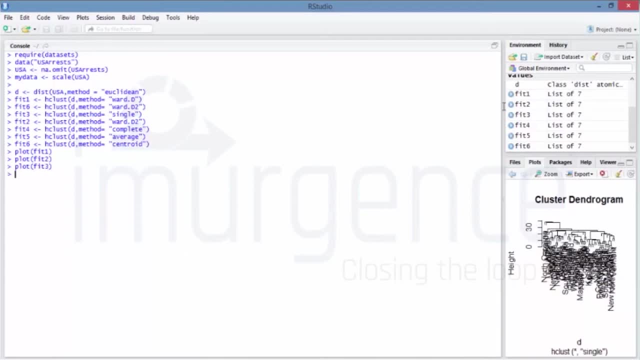 will be a little bit of difference in each of these which will fit three, if each of these which will fit three, if each of these which will fit three, if you can see the scale has changed. you can see the scale has changed. you can see the scale has changed drastically and the whole structure of 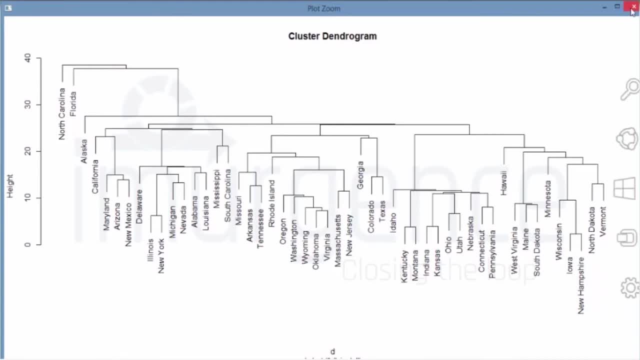 drastically and the whole structure of drastically and the whole structure of the dendrogram has changed right. what was the dendrogram has changed right. what was the dendrogram has changed right. what was looking very flat over there, it's looking very flat over there. it's looking very flat over there. it's looking comparatively very different over. 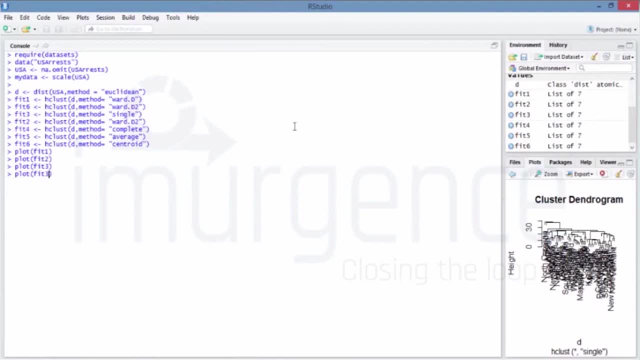 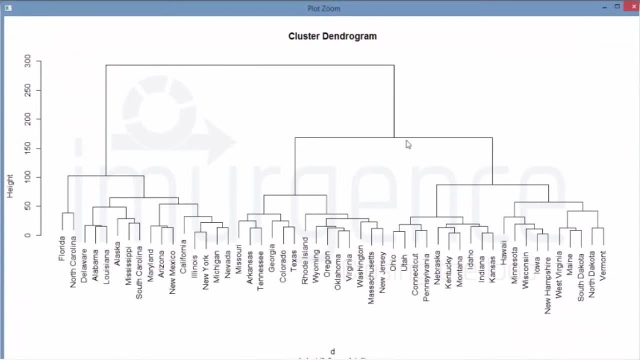 looking comparatively very different over looking comparatively very different over here. and do it for: also again: it's here. and do it for: also again it's here. and do it for also again: it's different from the previous one. this is different from the previous one. this is. 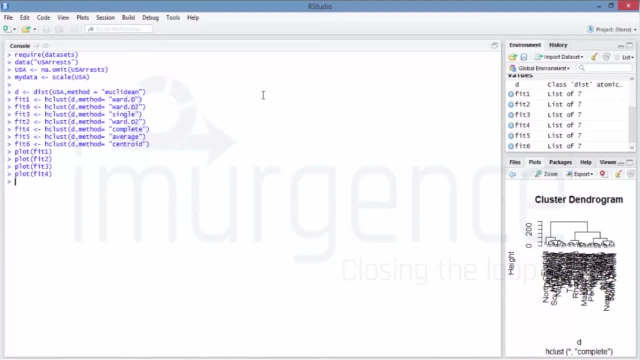 different from the previous one. this is because of the matrix method. whether because of the matrix method, whether because of the matrix method, whether you're using the central, the, the you're using the central, the, the you're using the central, the, the centroid method. whether you're using the. 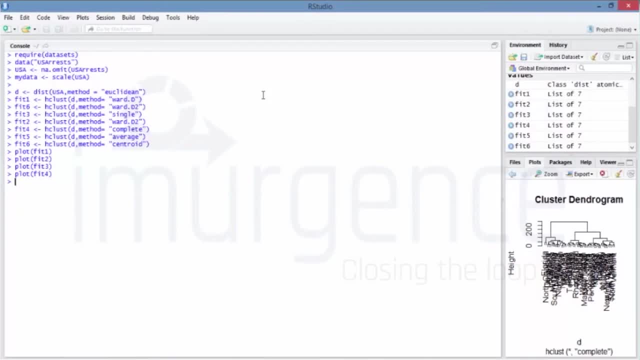 centroid method, whether you're using the centroid method, whether you're using the single linkage right, all those things, single linkage right. all those things, single linkage right. all those things. because of this, because of this, because of this, it's changing. so you can again do for it's changing, so you can again do for. 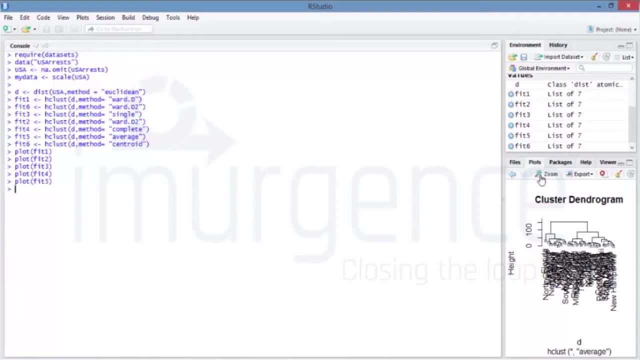 it's changing. so you can again do for the fifth one also, and for now you can the fifth one also, and for now you can the fifth one also, and for now you can bunch up these things and I can say: bunch up these things, and I can say: 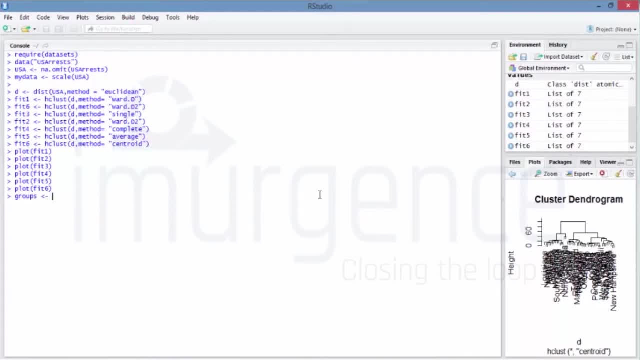 bunch up these things and I can say: groups location sign- cut tree dalgona. groups location sign- cut tree dalgona. groups location sign- cut tree dalgona- from itself. so you're saying fit one. so from itself. so you're saying fit one. so from itself. so you're saying fit one. so what you're trying to do is you're just 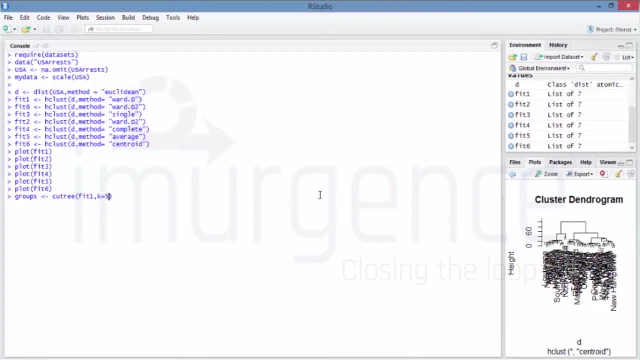 what you're trying to do is you're just what you're trying to do is you're just trying to do some housekeeping over here, trying to do some housekeeping over here, trying to do some housekeeping over here. so you're basically cutting it to five. 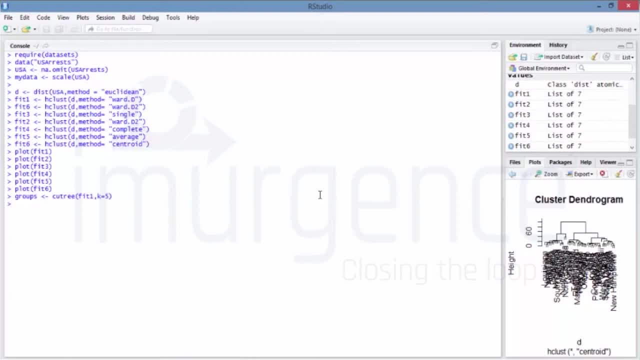 so you're basically cutting it to five. so you're basically cutting it to five clusters, and that's also something you clusters, and that's also something you clusters and that's also something you can do. have a look at this also. get the can do. have a look at this also. get the. 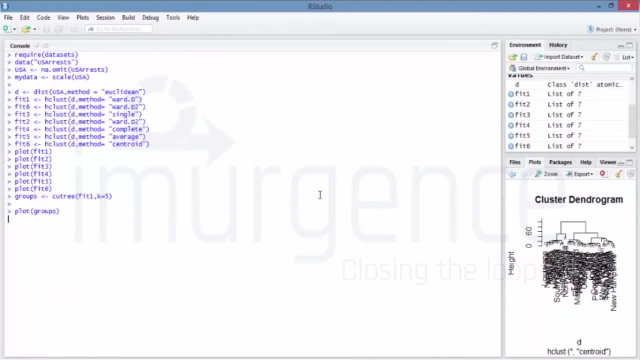 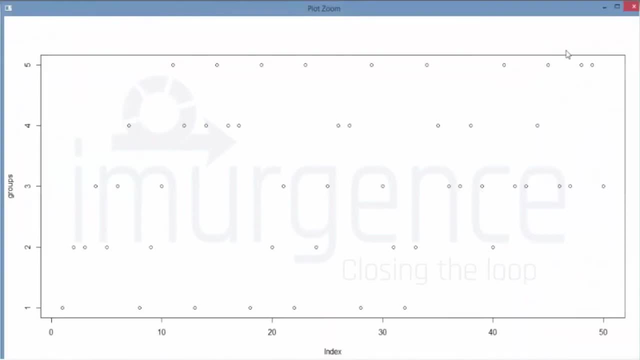 can do. have a look at this also. get the plot can do this way also. just chopping plot can do this way also. just chopping plot can do this way also, just chopping it off. so now I'm using rect dot it off. so now I'm using rect dot. 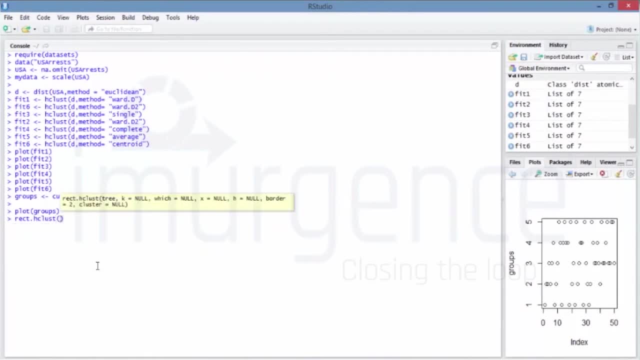 it off. so now I'm using rect dot H classed and that I'm passing fit one H classed and that I'm passing fit one H classed and that I'm passing fit one. I'm saying number of clusters has to be. I'm saying number of clusters has to be. 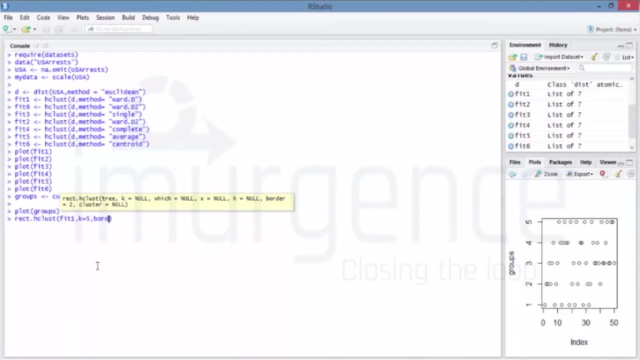 I'm saying: number of clusters has to be fine and the color border color has to fine and the color border color has to fine and the color border color has to be correct. so that's what you're doing: be correct. so that's what you're doing. 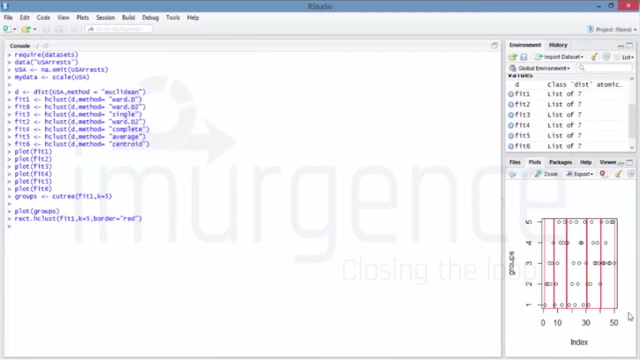 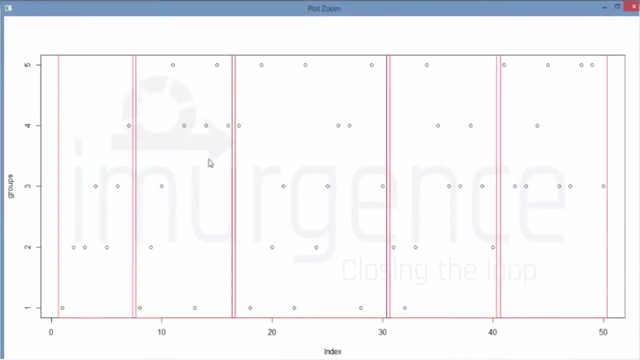 be correct. so that's what you're doing over here. these are the groups. I'm just over here. these are the groups. I'm just over here. these are the groups. I'm just zooming this so that you can have a look. zooming this so that you can have a look. 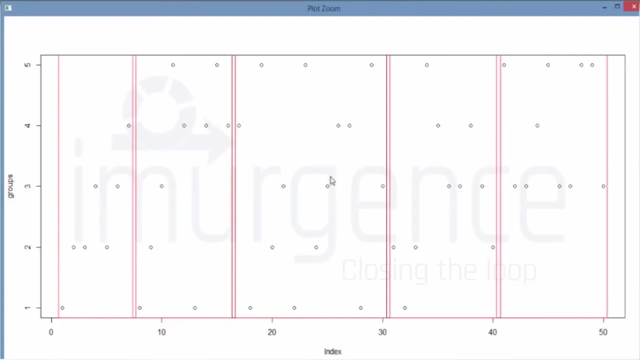 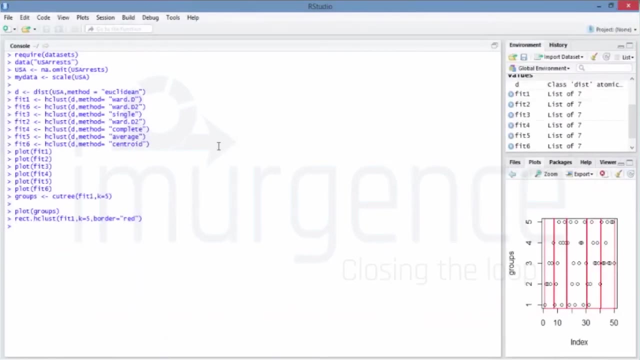 zooming this so that you can have a look. so you are basically partitioned into. so you are basically partitioned into. so you are basically partitioned into different bases. this value, so you have different bases. this value, so you have different bases, this value. so you have just partitioned this. so, as you can see, 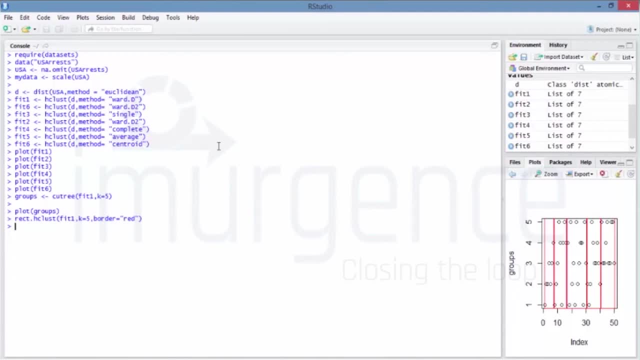 just partitioned this so, as you can see, just partitioned this. so, as you can see, on the screen, it's showing the same on the screen. it's showing the same on the screen. it's showing the same picture. so it didn't picture, so it didn't. 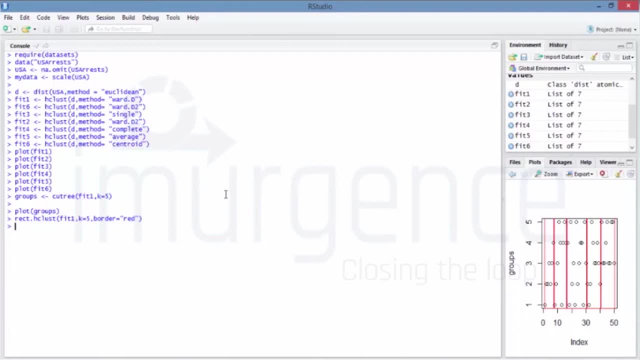 picture, so it didn't. endogram of agglomerative hierarchical endogram of agglomerative hierarchical endogram of agglomerative hierarchical clustering as grouped into five clusters. clustering as grouped into five clusters. clustering as grouped into five clusters. that's what we can see. now there is a. 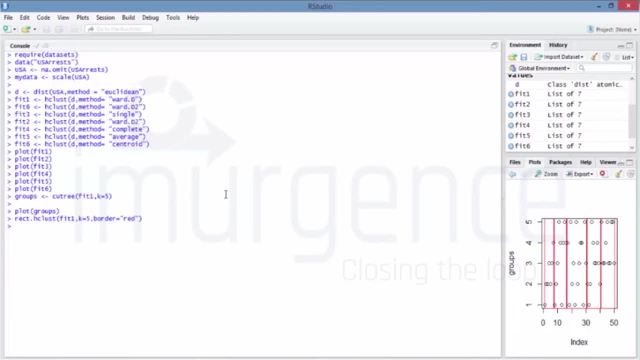 that's what we can see now. there is a- that's what we can see now. there is a function called SPV cluster in the PV function called SPV cluster in the PV function called SPV cluster in the PV cluster package, which provides P values. cluster package, which provides P values. 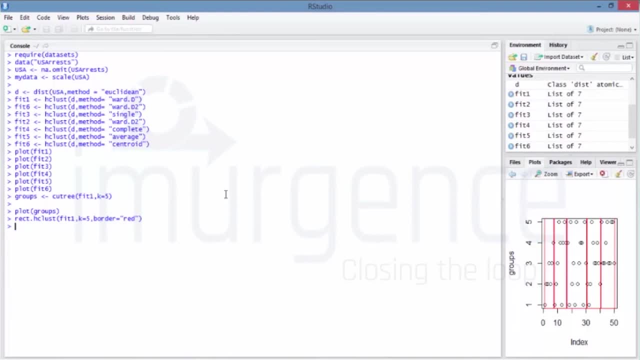 cluster package which provides P values for hierarchical clustering based on: for hierarchical clustering based on: for hierarchical clustering based on multi-scale bootstrap resampling. so multi-scale bootstrap resampling, so multi-scale bootstrap resampling. so, obviously, when you talk about, obviously, when you talk about, obviously, when you talk about bootstrapping, that means you are doing. 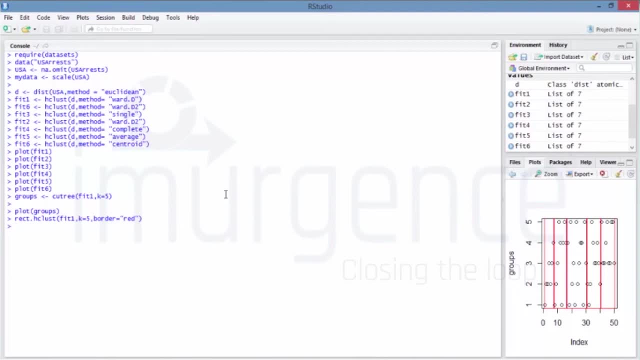 bootstrapping. that means you are doing bootstrapping. that means you are doing like keeping extracting the same data, like keeping extracting the same data, like keeping extracting the same data again and again from a whole set of again and again from a whole set of again and again from a whole set of population, randomly, and you are allowing. 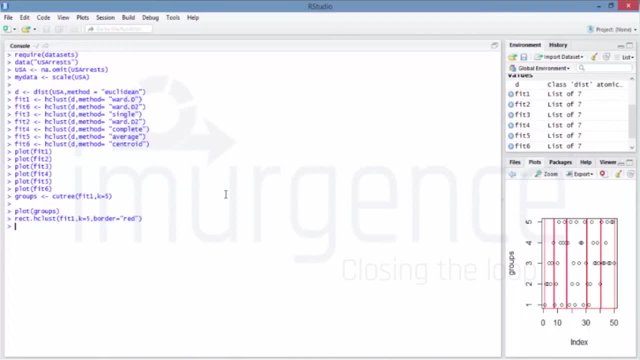 population randomly and you are allowing population randomly and you are allowing. replace is equal to true. that means the replace is equal to true. that means the replace is equal to true. that means the same observation might be picked up more. same observation might be picked up more. same observation might be picked up more than once. now you are doing this in. 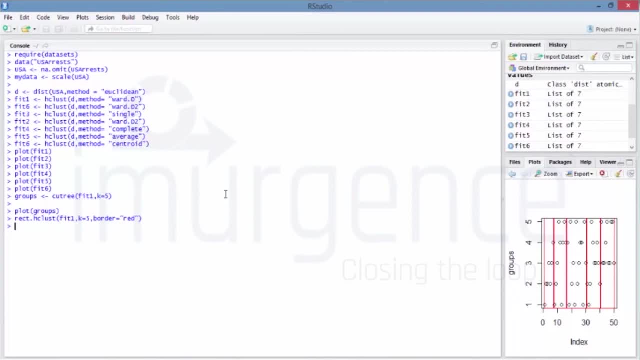 than once now you are doing this, in than once now you are doing this in absence of exposure to complete, absence of exposure to complete, absence of exposure to complete population available to you, so that this population available to you, so that this population available to you, so that this sample which you're extracting is. 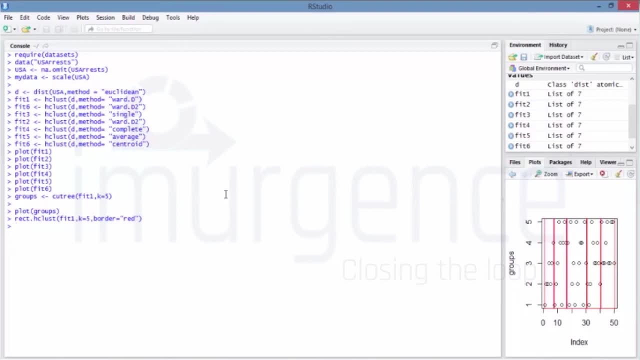 sample which you're extracting is sample which you're extracting is somewhere becoming closer to the real, somewhere becoming closer to the real, somewhere becoming closer to the real population. that is what the concept of population, that is what the concept of population, that is what the concept of bootstrapping is right. so these clusters, 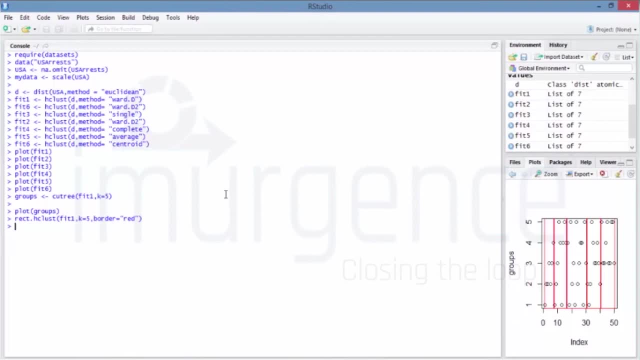 bootstrapping is right. so these clusters: bootstrapping is right. so these clusters are highly supported by the data, which are highly supported by the data, which are highly supported by the data which have larger p-values. right, but you have have larger p-values, right, but you have. 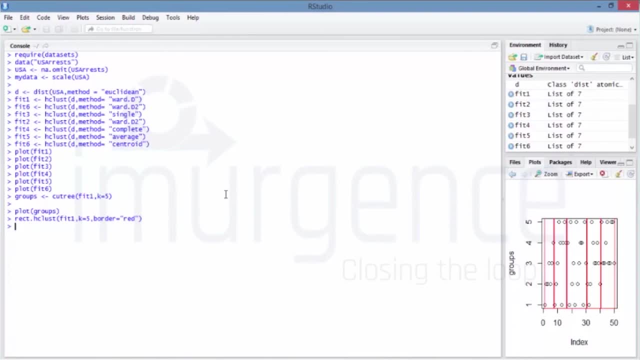 have larger p-values, right, but you have to be very aware that the TV class to be very aware that the TV class to be very aware that the TV class clusters columns, not rows. so you have to clusters columns, not rows. so you have to clusters columns, not rows. so you have to transpose your data before using them. 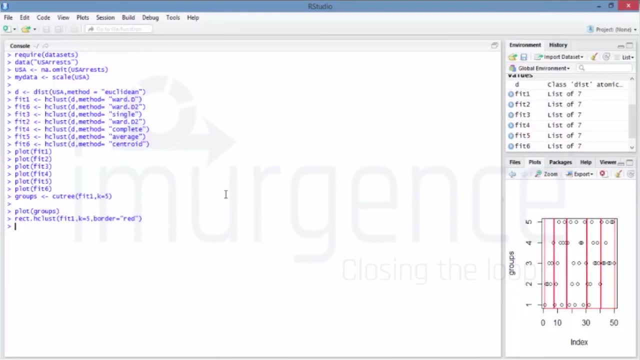 transpose your data before using them. transpose your data before using them, right? so traditionally, what happens? your right. so traditionally, what happens? your right, so traditionally, what happens: your data is kept as a column. so, based on data is kept as a column. so, based on data is kept as a column. so based on that, the clustering happens. but this: 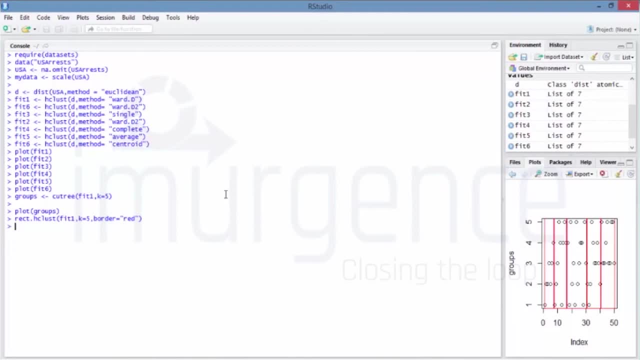 that the clustering happens, but this: that the clustering happens. but this specific algorithm works on rows. rather specific algorithm works on rows. rather specific algorithm works on rows rather than columns. so you'll have to transpose than columns. so you'll have to transpose than columns. so you'll have to transpose your data before you go ahead and do. 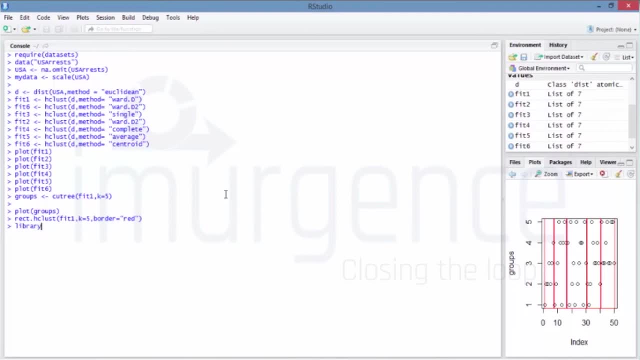 your data before you go ahead and do your data, before you go ahead and do this processing. so first of all, you have this processing. so first of all, you have this processing. so first of all, you have to install this package and then load. to install this package and then load. 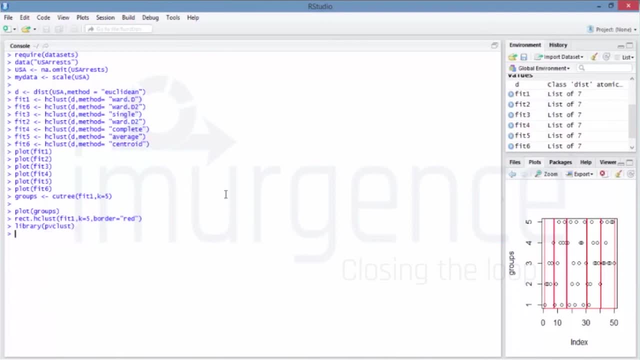 to install this package and then load TV cluster package, and then you will just TV cluster package, and then you will just TV cluster package, and then you will just say something like a fifth allocation. say something like a fifth allocation, say something like a fifth allocation, sign TV cluster, which then you're going. 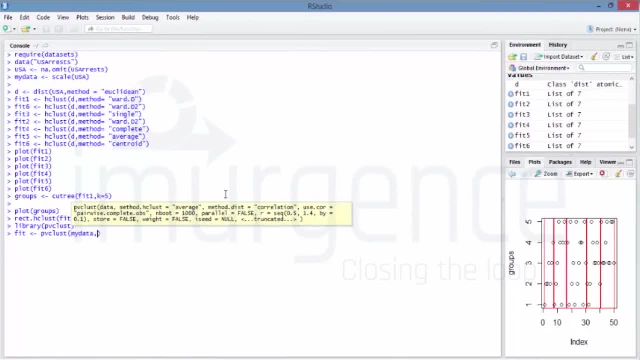 sign TV cluster which then you're going sign TV cluster, which then you're going to call your data. we have already saved to call your data. we have already saved to call your data. we have already saved that in my data. if you remember, we had that in my data. if you remember, we had. 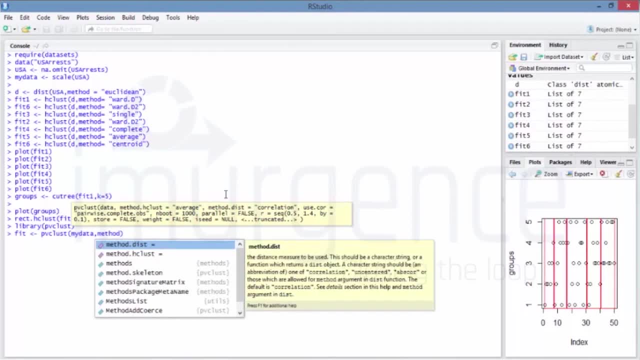 that in my data, if you remember we had done that scaling work. then we say: done that scaling work. then we say: done that scaling work. then we say: method dot. edge clust is equal to ward. method dot. edge clust is equal to ward. method dot. edge clust is equal to ward. it's name of the scientist and method. 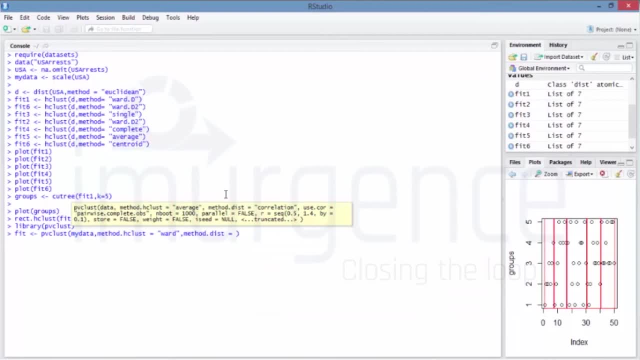 it's name of the scientist and method. it's name of the scientist and method: dot distance computation. is you dot distance computation? is you dot distance computation? is you clearly, clearly, clearly, right, right, right? so it says that the ward method has. so it says that the ward method has. 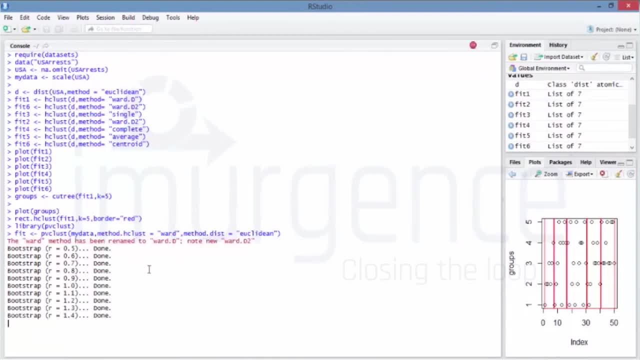 so it says that the ward method has been replaced to ward dot be, so it has done. been replaced to ward dot be, so it has done. been replaced to ward dot be, so it has done that automatically. and these are the that automatically, and these are the that automatically, and these are the bootstrappings which has been internal. 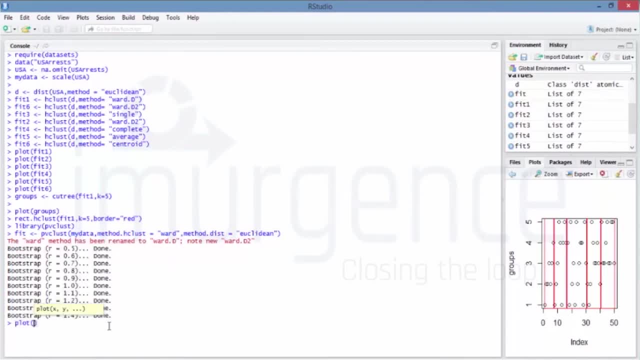 bootstrappings which has been internal bootstrappings, which has been internal done, and then we can do a plot of this done, and then we can do a plot of this done, and then we can do a plot of this plot of set. so here you have your. 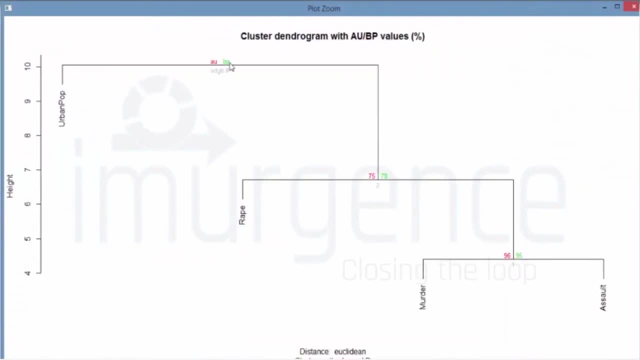 plot of set. so here you have your plot of set. so here you have your diagram diagram. diagram diagram: the analysis of what is the output is shown. the analysis of what is the output is shown. the analysis of what is the output is shown on the next screen when we'll have a. 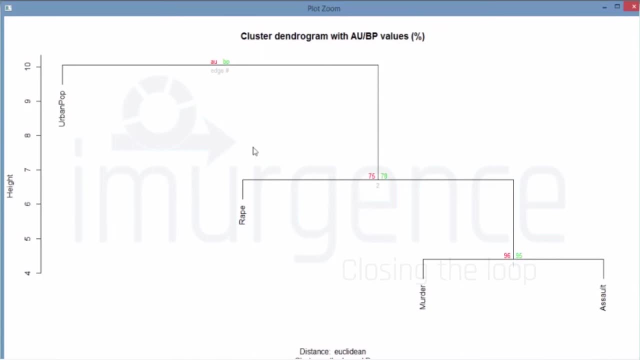 on the next screen, when we'll have a on the next screen, when we'll have a. look at this picture. this is your output. look at this picture. this is your output. look at this picture. this is your output. this is the height. this is the urban. this is the height. this is the urban. 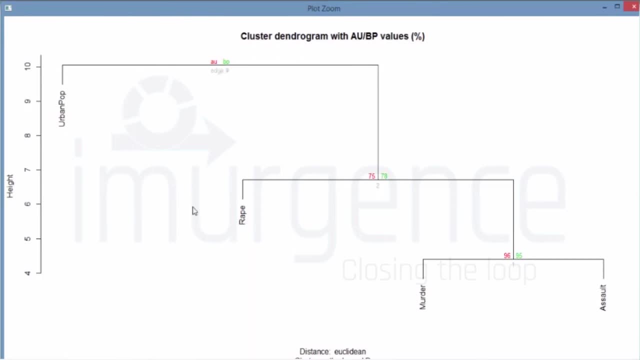 this is the height. this is the urban population. this is talking about a population. this is talking about a population. this is talking about a variable: the percentage of rape over your variable. the percentage of rape over your variable. the percentage of rape over your percentage of murder and assault right. 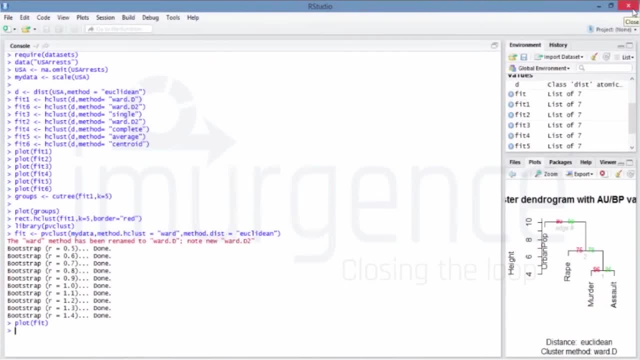 percentage of murder and assault right. percentage of murder and assault right. you'll have a look at this on the screen. you'll have a look at this on the screen. you'll have a look at this on the screen, and just on the previous screen, if you, and just on the previous screen, if you. 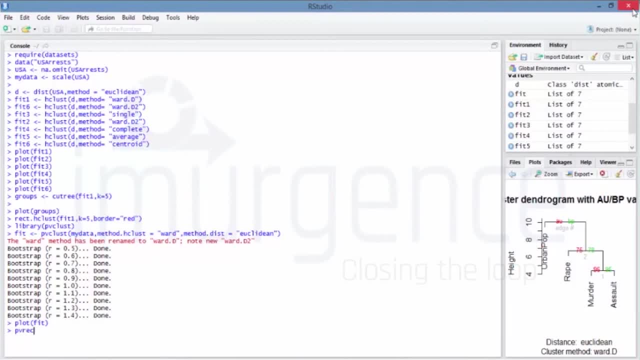 and just on the previous screen, if you can see there is something called as PV, can see there is something called as PV, can see there is something called as PV direct right, which is an additional direct right, which is an additional direct right, which is an additional parameter. if you want to check and you 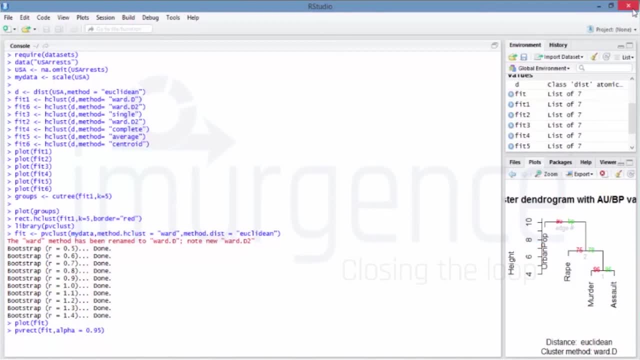 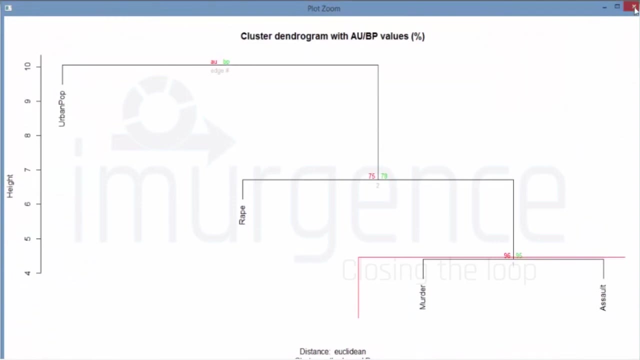 parameter if you want to check, and you parameter if you want to check, and you giving the confidence interval over here, giving the confidence interval over here, giving the confidence interval over here. so it's so, it's so, it's okay, okay, okay. so what is basically? PV cluster, PV class? 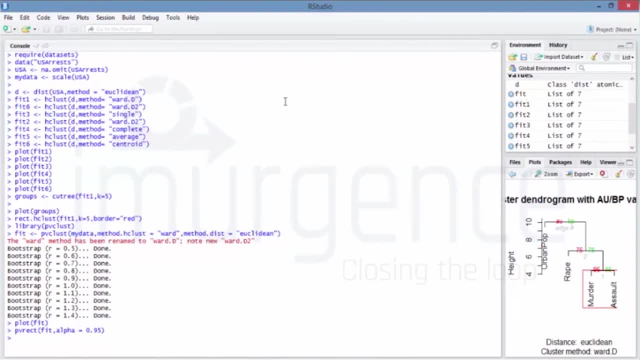 so what is basically PV cluster PV class? so what is basically PV cluster? PV class provides two types of p-values: au. that is, provides two types of p-values. au. that is, provides two types of p-values. au. that is approximately unbiased, which you had, approximately unbiased, which you had. 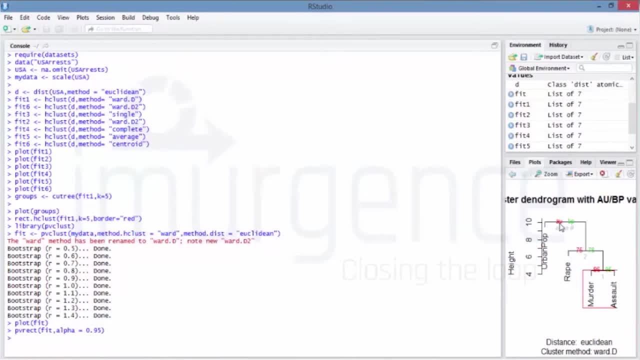 approximately unbiased, which you had seen over here au unbiased p-value and seen over here au unbiased p-value and seen over here au unbiased p-value and BP, that is the bootstrapped probability. BP, that is the bootstrapped probability. BP, that is the bootstrapped probability values. obviously, when you're when you 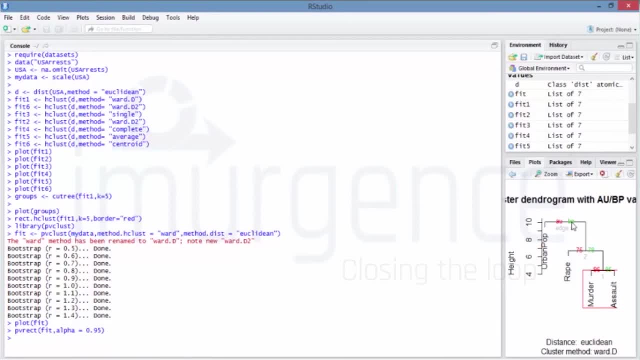 values. obviously when you're when you values, obviously when you're when you talk about something like decision tree, talk about something like decision tree. talk about something like decision tree. all those things bootstrapped is a good. all those things bootstrapped is a good. all those things bootstrapped is a good thing to look at. right the au value. 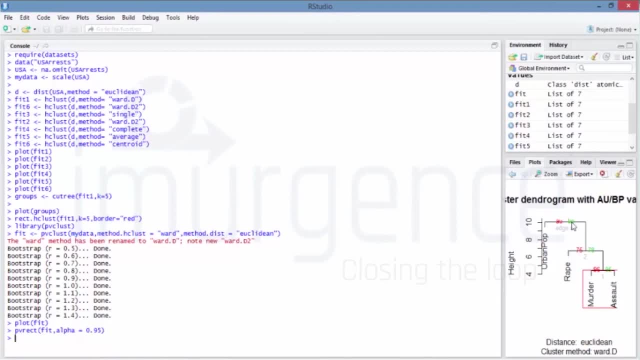 thing to look at right: the au value thing to look at right: the au value which is computed by multi-scale, which is computed by multi-scale, which is computed by multi-scale. bootstrap resampling is a better bootstrap resampling is a better bootstrap resampling is a better approximation to unbiased p-value. then 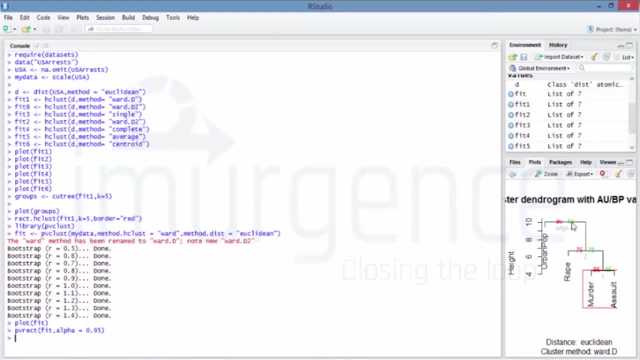 approximation to unbiased p-value. then approximation to unbiased p-value, then BP value computed by normal bootstrap BP value computed by normal bootstrap BP value computed by normal bootstrap resampling right. so it says that the au resampling right. so it says that the au resampling right. so it says that the au, that is, the unbiased p-value, is a far. 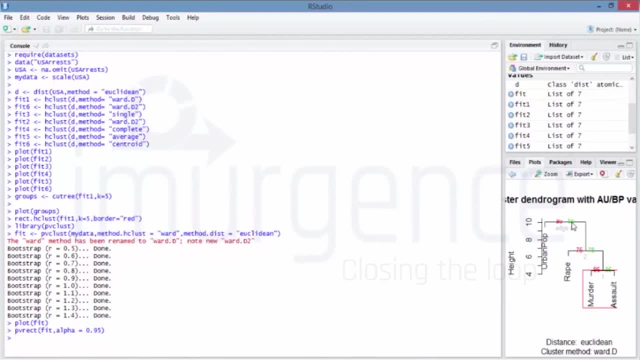 that is the unbiased p-value, is a far, that is the unbiased p-value, is a far better method of approximating to. the better method of approximating to: the better method of approximating to the unbiased p-value, then BP value computed. unbiased p-value, then BP value computed. 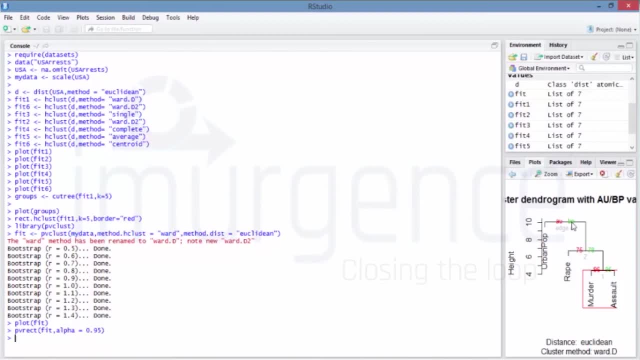 unbiased p-value, then BP value computed by normal bootstrap resampling. but if by normal bootstrap resampling, but if by normal bootstrap resampling, but if you are a person who is into machine, you are a person who is into machine. you are a person who is into machine learning, you might yourself get into the. 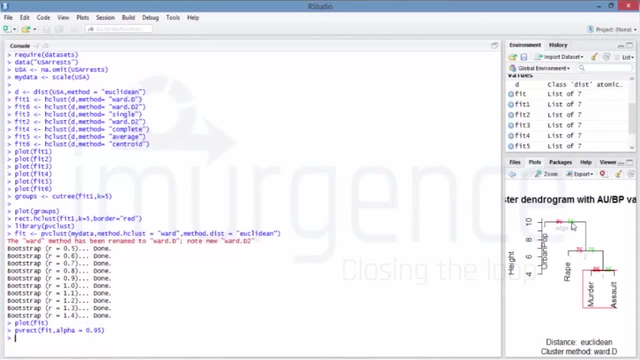 learning. you might yourself get into the learning. you might yourself get into the bootstrapping aspect and create a bootstrapping aspect and create a bootstrapping aspect and create a decision tree, which is which you can, decision tree, which is which you can, decision tree, which is which you can control. PV class performs hierarchical. 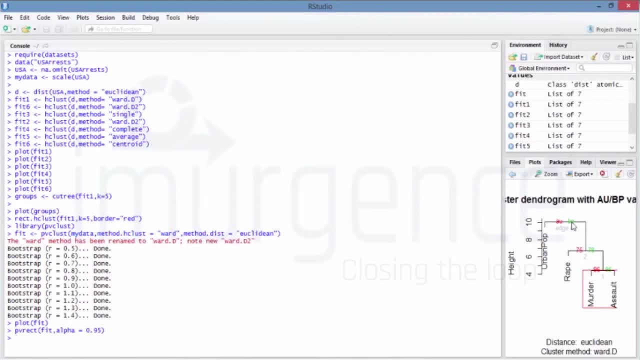 control. PV class performs hierarchical control. PV class performs hierarchical cluster analysis by a function H, cluster analysis by a function H. cluster analysis by a function H classed and automatically computes the classed. and automatically computes the classed and automatically computes the p-values for all the clusters. constraint. 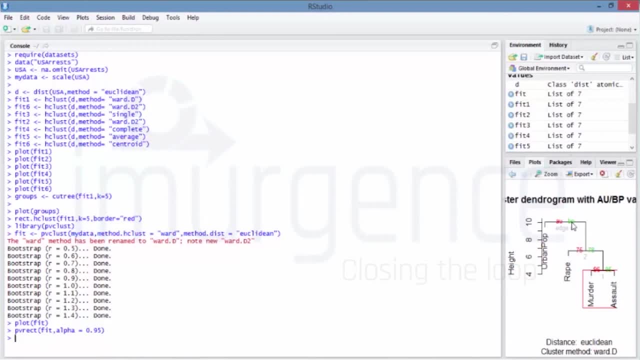 p-values for all the clusters. constraint. p-values for all the clusters. constraint: contained in the clustering of original. contained in the clustering of original. contained in the clustering of original data. right? so it will do the hierarchical data right. so it will do the hierarchical data right. so it will do the hierarchical cluster analysis via the H class. so you. 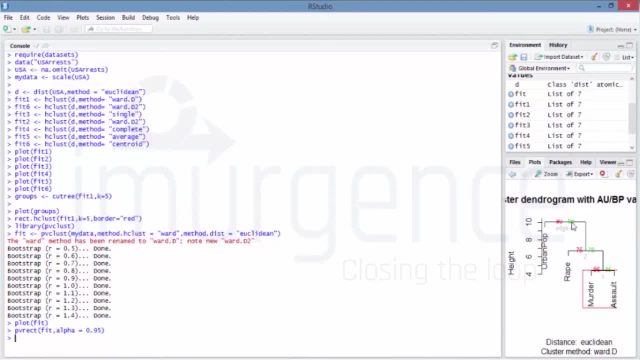 cluster analysis via the H class. so you cluster analysis via the H class. so you have used the edge cluster prior to this. have used the edge cluster prior to this, have used the edge cluster prior to this. right, so the PV cluster is going to call. right, so the PV cluster is going to call. 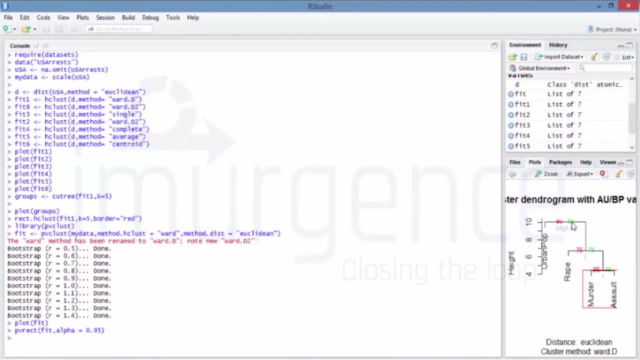 right, so the PV cluster is going to call the same function and it computes the the same function and it computes the the same function and it computes the clusters, but it gives importance to clusters. but it gives importance to clusters, but it gives importance to significance test, whereas in the prior 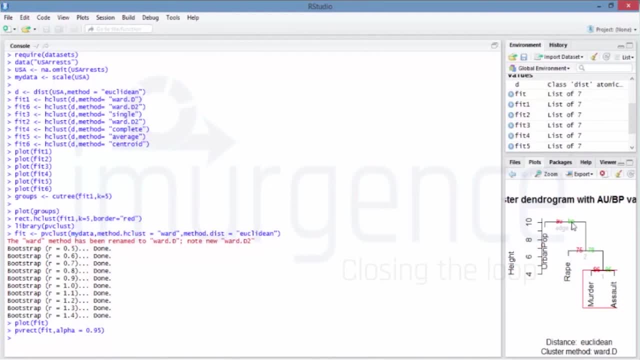 significance test. whereas in the prior significance test, whereas in the prior case the p-values were not considered case, the p-values were not considered case. the p-values were not considered. over here the p-values are considered as over here the p-values are considered as over here the p-values are considered as part of the cluster formation process. it 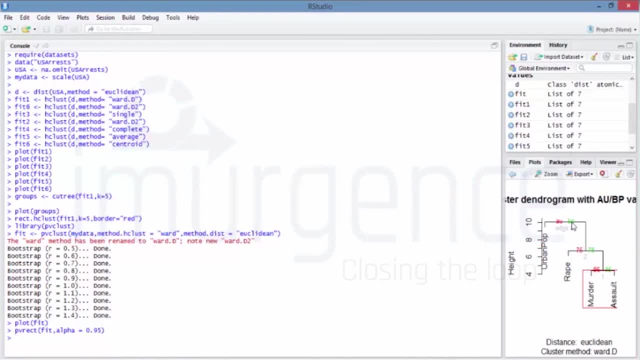 part of the cluster formation process. it part of the cluster formation process. it also provides graphical tools, such as: also provides graphical tools, such as: also provides graphical tools, such as plot function or useful TV rect function. plot function or useful TV rect function. plot function or useful TV rect function, which highlights clusters with. 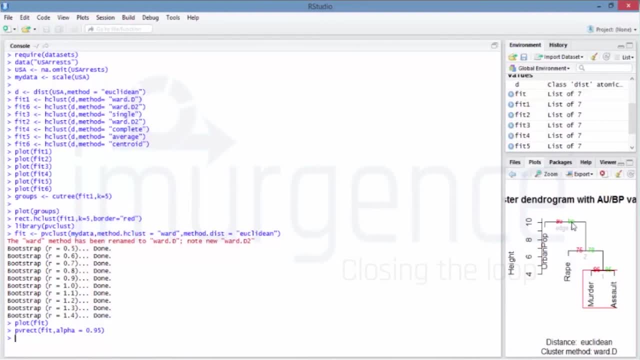 which highlights clusters with which highlights clusters with relatively high or relatively very low, relatively high or relatively very low, relatively high or relatively very low p-value. so it's just a way of redrawing p-value. so it's just a way of redrawing p-value, so it's just a way of redrawing it again. so importance or importance can. 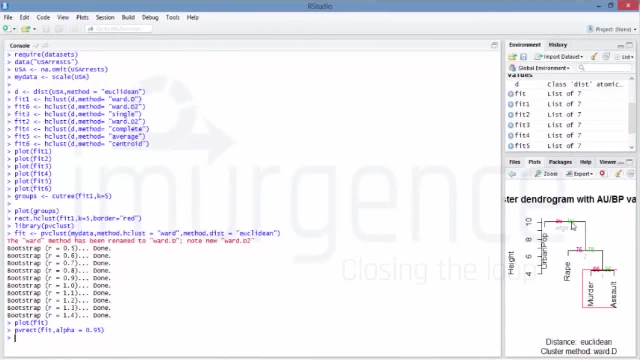 it again. so importance or importance, can it again. so importance or importance can be given to extreme p-values- right so to be given to extreme p-values, right so to be given to extreme p-values, right so to highlight them. now you have an example, highlight them. now you have an example. 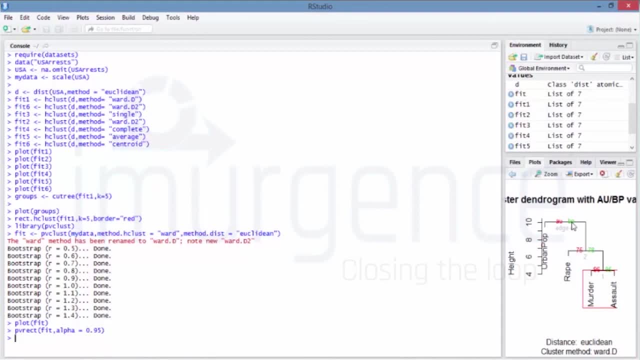 highlight them. now you have an example: or when we will be using the PV cluster, or when we will be using the PV cluster, or when we will be using the PV cluster again. so in this case, we are again going again. so in this case, we are again going. 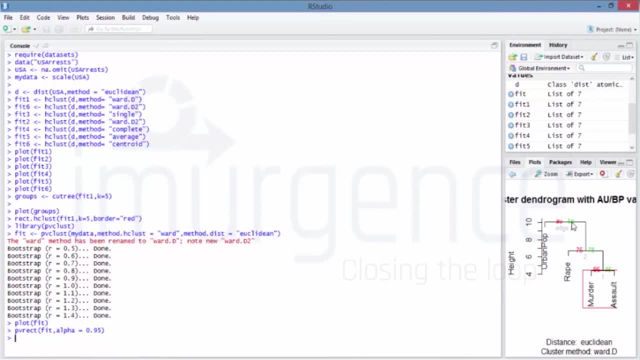 again. so in this case we are again going to call the same data. right the USA to call the same data. right the USA to call the same data. right the USA data. but it's not the scale data, so I'm data, but it's not the scale data, so I'm. 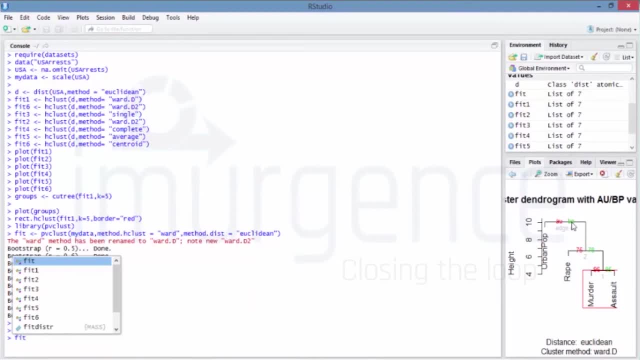 data, but it's not the scale data. so I'm going to best pass that into fit 7, going to best pass that into fit 7, going to best pass that into fit 7, because we had done till fit fit 6, so an. because we had done till fit fit 6, so an. 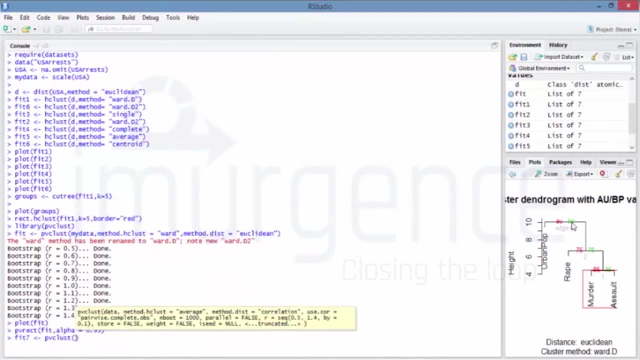 because we had done till fit fit 6, so an extension. so we say PV cluster bracket extension. so we say PV cluster bracket extension. so we say PV cluster bracket class. USA method dot edge clust. if you class USA method dot edge clust. if you class USA method dot edge clust. if you remember, we had shared over there that 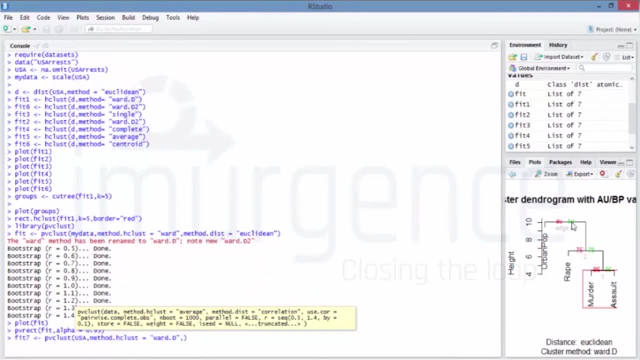 remember we had shared over there that. remember we had shared over there that ward dot D could be the output. because ward dot D could be the output, because ward dot D could be the output, because it has been renamed to this comma method. it has been renamed to this comma method. 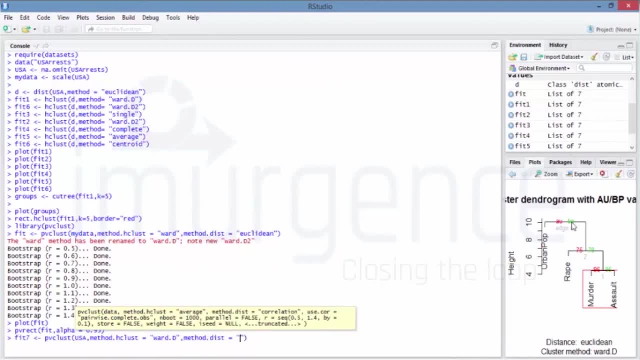 it has been renamed to this comma method: dot distance is equal to u CLI de en dot distance is equal to u CLI de en dot distance is equal to u CLI de en Euclidean, and yes, you will just run. Euclidean, and yes, you will just run. 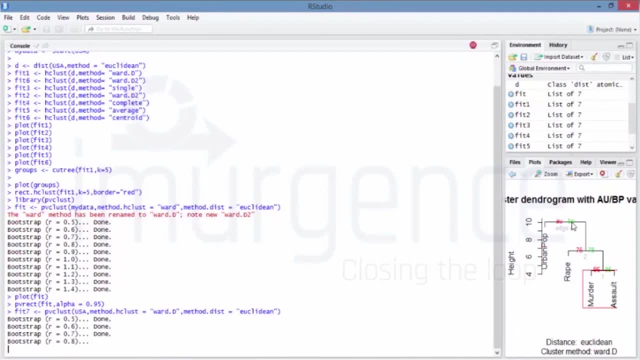 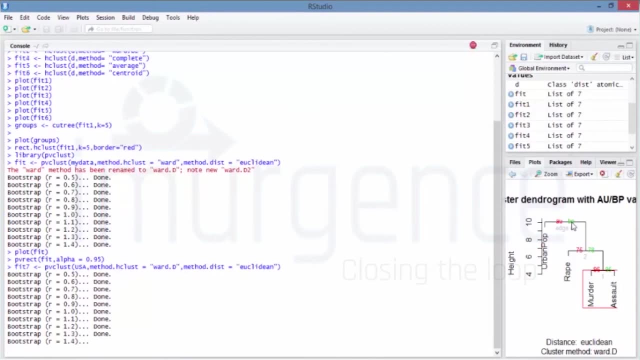 Euclidean, and yes, you will just run this into the bootstrapping for you, first this into the bootstrapping for you, first this into the bootstrapping for you, first right and after this you can just do a right and after this you can just do a. 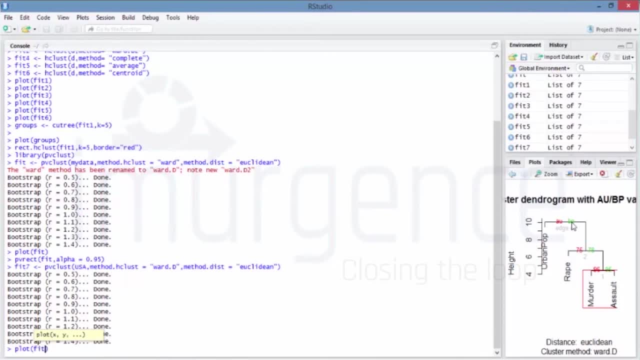 right, and after this you can just do a plot of the same again. so just doing that plot of the same again. so just doing that plot of the same again. so just doing that again. you get the dendrogram bit to. again you get the dendrogram bit to. 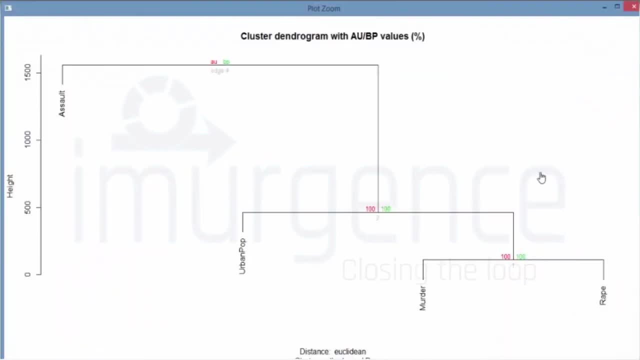 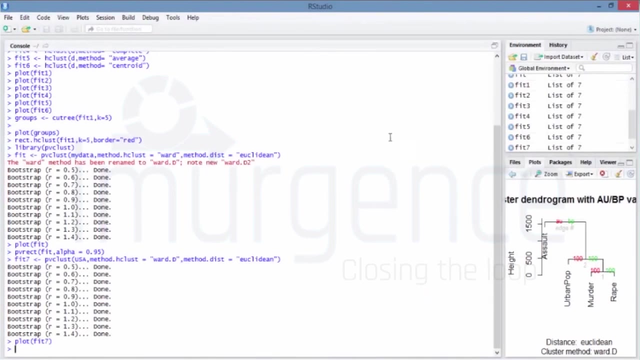 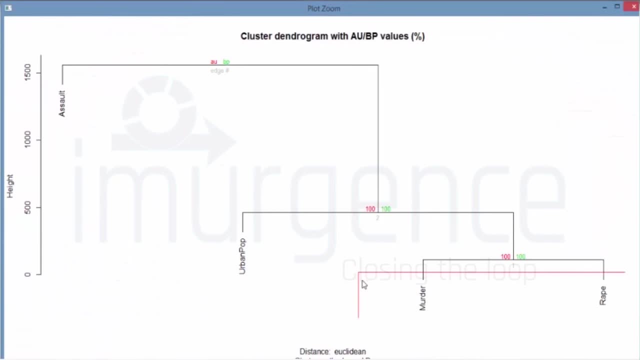 alpha is equal to 0.95, right, so you can. alpha is equal to 0.95, right, so you can see this highlight which has happened. see this highlight which has happened. see this highlight which has happened over here. obviously you cannot see the over here, obviously you cannot see the. 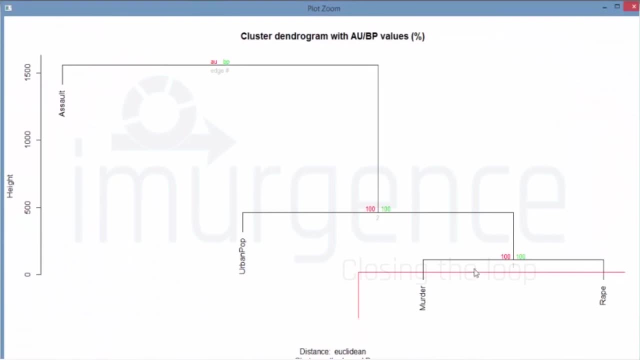 over here. obviously you cannot see the box, but this ideally creating a box over box, but this ideally creating a box over box, but this ideally creating a box over here which you can see to a certain here, which you can see to a certain here, which you can see to a certain extent when you're so, you're seeing it. 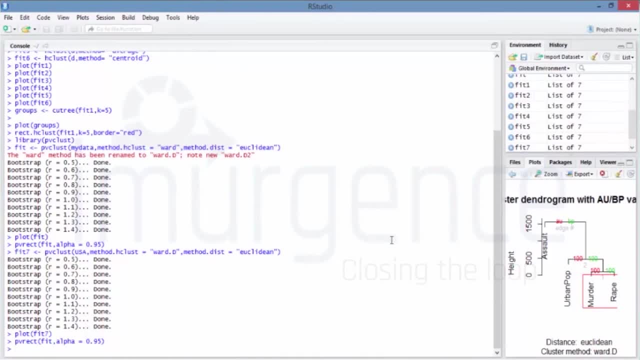 extent when you're so, you're seeing it. extent when you're so, you're seeing it over here because, as you're expanding, are over here, because, as you're expanding, are over here because, as you're expanding, are is not able to show it properly, so is not able to show it properly. so. 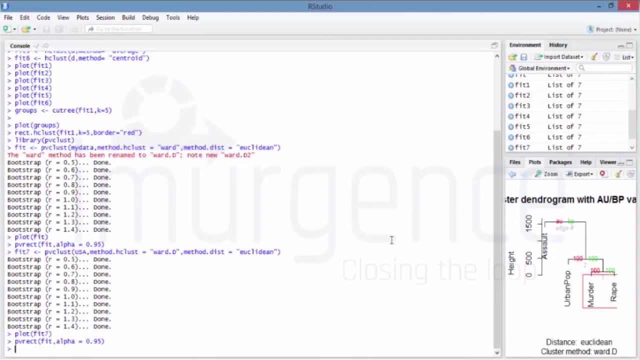 is not able to show it properly, so the highlighted portion is shown over here. the highlighted portion is shown over here. the highlighted portion is shown over here. the values of the edges of the. the values of the edges of the. the values of the edges of the clustering are P values, basically. 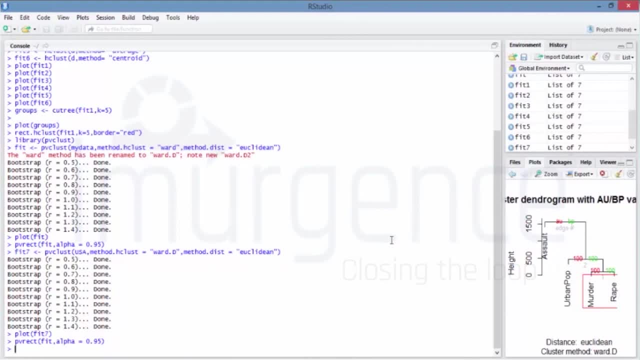 clustering are P values basically. clustering are P values basically percentages if you multiply by 100, and percentages if you multiply by 100. and percentages if you multiply by 100 and the red values are the AUP values right? the red values are the AUP values right. 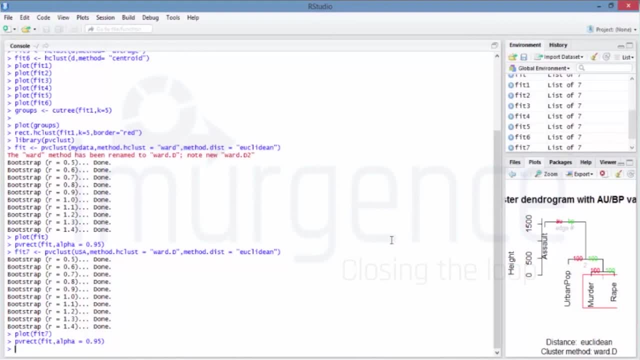 the red values are the AUP values right and the green values are the bootstrap and the green values are the bootstrap and the green values are the bootstrap values. clusters with a you larger than values, clusters with a you larger than values, clusters with a you larger than 95% are highlighted by rectangles, which. 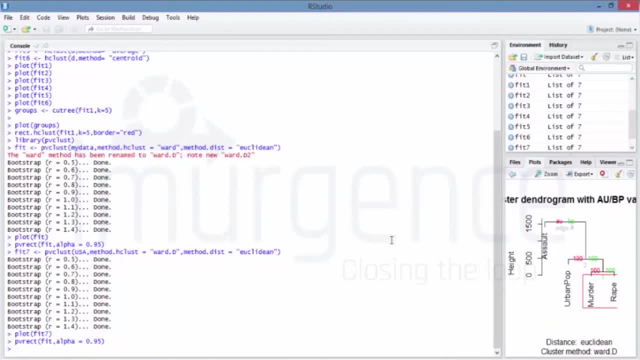 95% are highlighted by rectangles, which 95% are highlighted by rectangles, which are strongly supported by the data. so are strongly supported by the data, so are strongly supported by the data. so again, a significance test is done. and if, again a significance test is done, and if